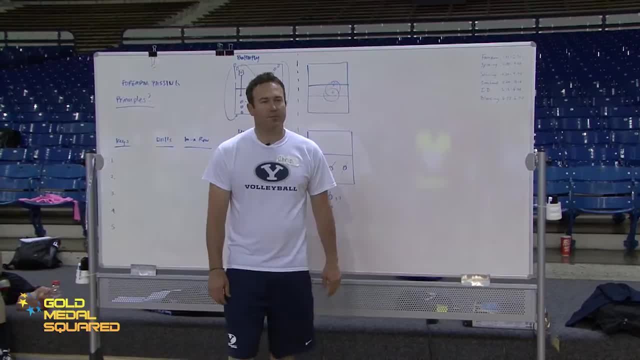 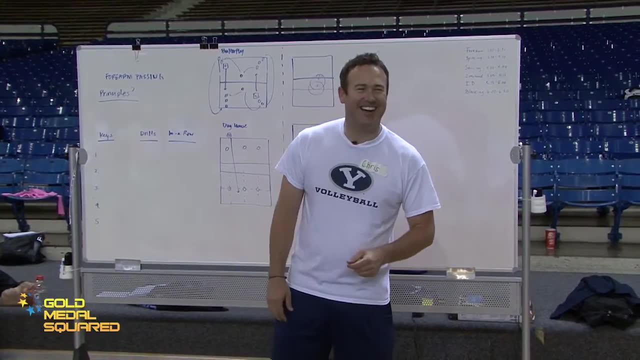 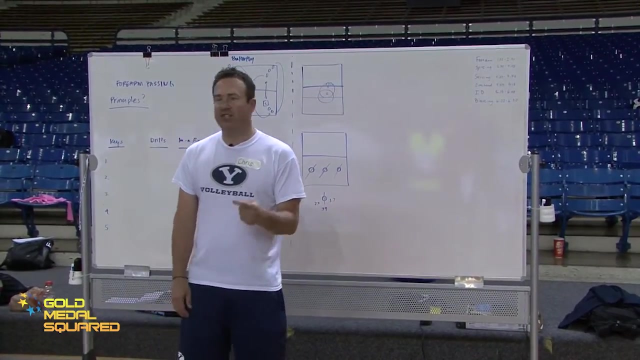 The same way. So, yeah, my motor program becomes good, nice and Shannon- look at her All right- And ultimately it increases our accuracy or our ability to execute that skill the same way over and over again, like we talked about that repeatability. So simplicity. 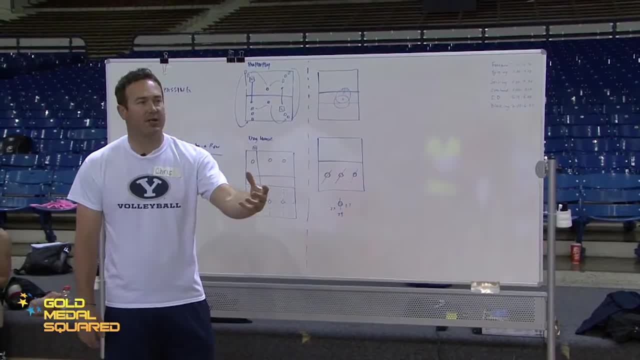 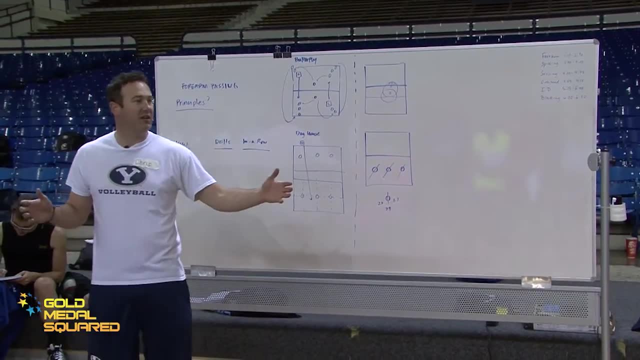 equals repeatability, equals accuracy, And so that's a principle that we'd like to create, this simple movement, And that's probably applies across any skill that we're going to do. but certainly, in passing, What's another principle that we talk about? 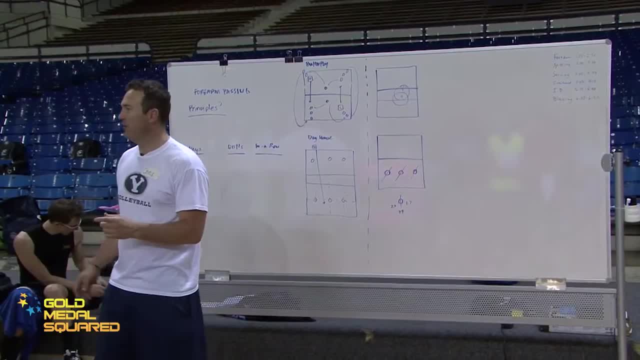 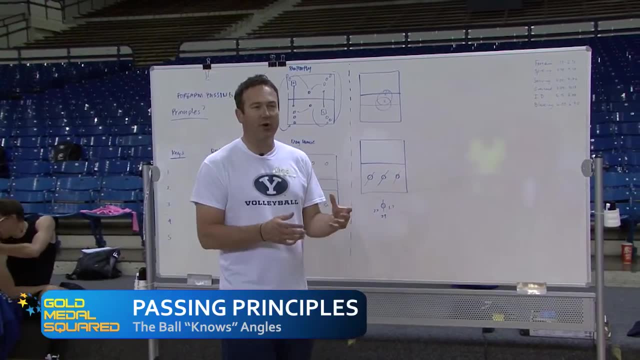 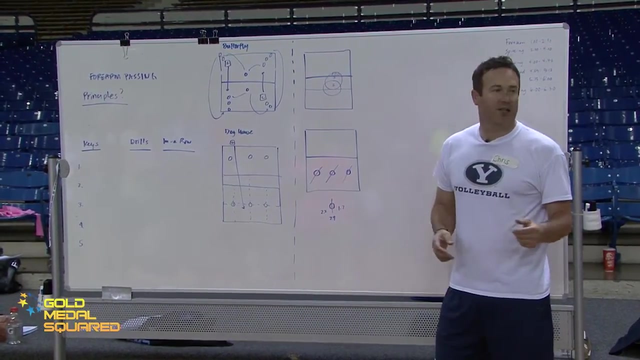 That's a key. So the ball knows angles is what we're going to say- And that's kind of a funny way to talk about it- that the ball knowing something. But the ball simply is going to behave based on these angles, And that makes sense, right? It's just going to obey the laws of physics here, basically, And so 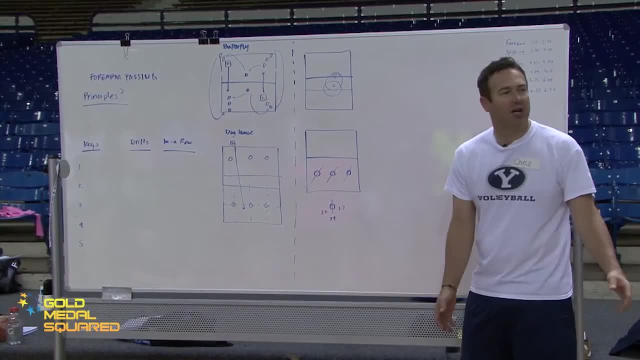 what we're trying to do is we're going to use the principle of being able to be based on these angles. And so what we're trying to do is we're going to use the principle of being able to be based on these angles to do is, manipulate or present a great angle for the ball to bounce off of. 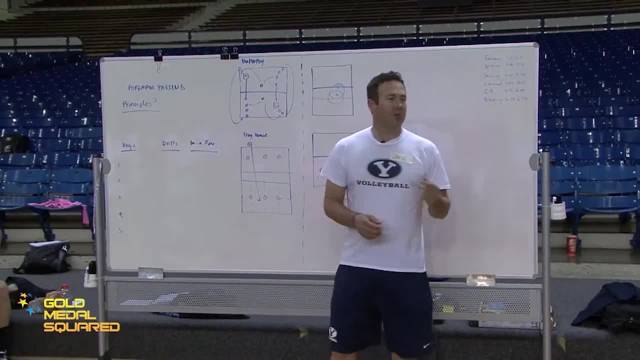 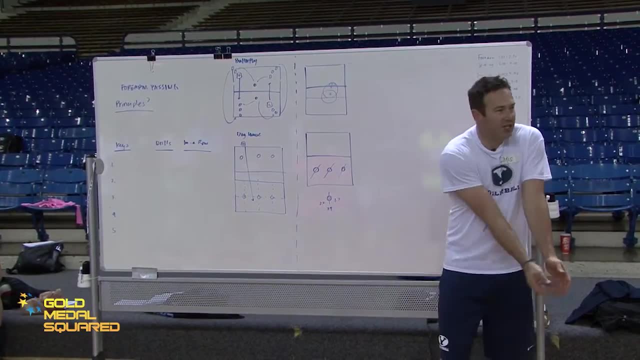 And we like to joke that the ball doesn't know if you're blonde or a brunette, it doesn't know if you have green eyes or blue eyes, it doesn't know if you're a boy or a girl. All it knows is: here's this angle and I'm going to bounce off of that angle. 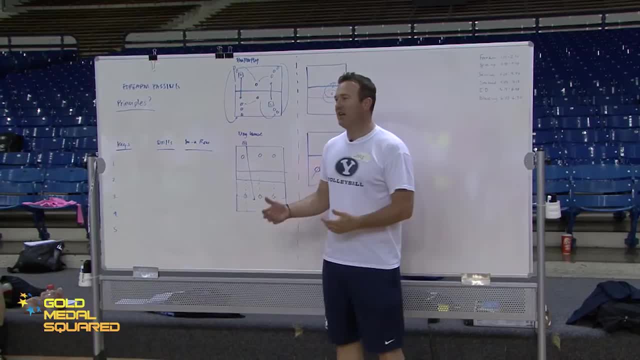 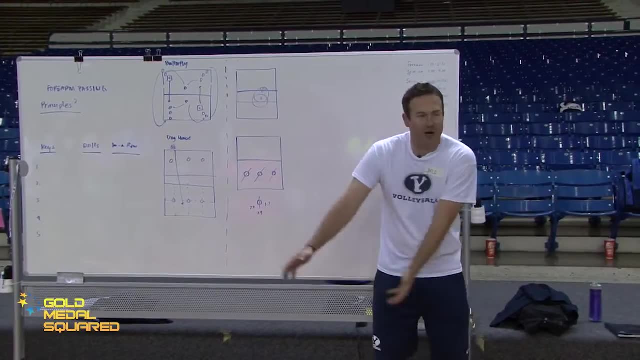 And if it was a good angle, it will bounce where we want it, and if it wasn't a good angle, it will obviously go somewhere else. And so that's kind of this idea that we're controlling the angle and we're trying to manipulate that angle. 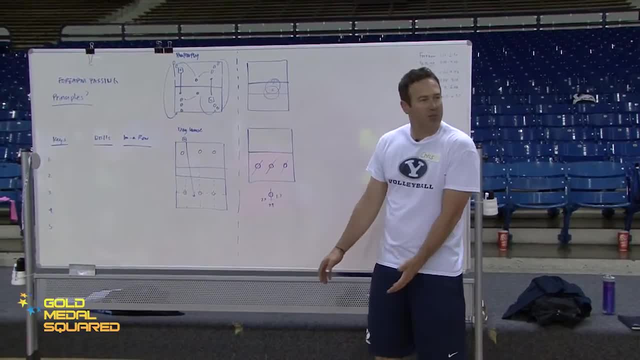 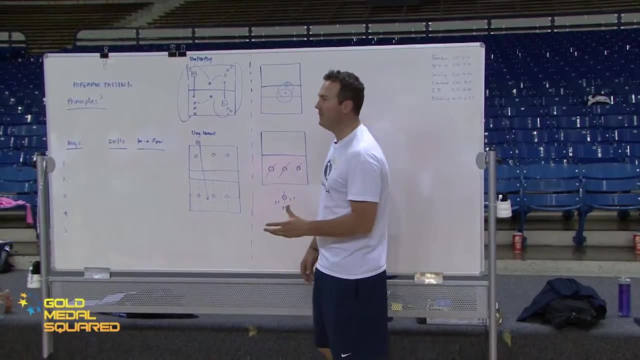 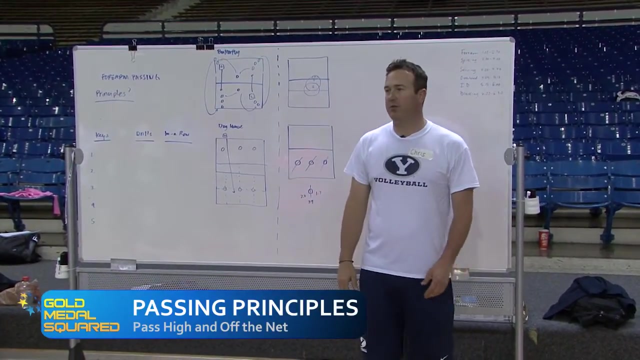 And so we want to move in ways that allow us to manipulate that angle and control that angle as efficiently as possible. What else Okay? so that's a nice principle that if we can keep things off the net, we're more likely to be able to play the ball on our side of the net, obviously. 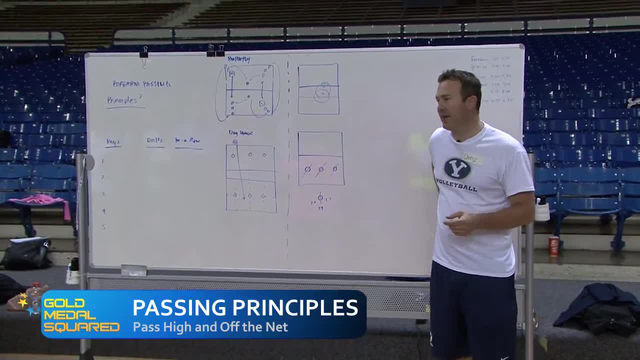 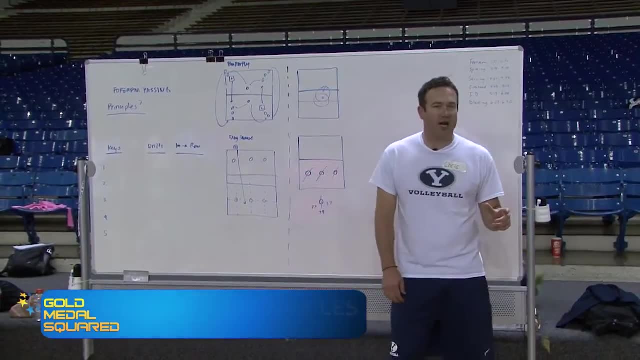 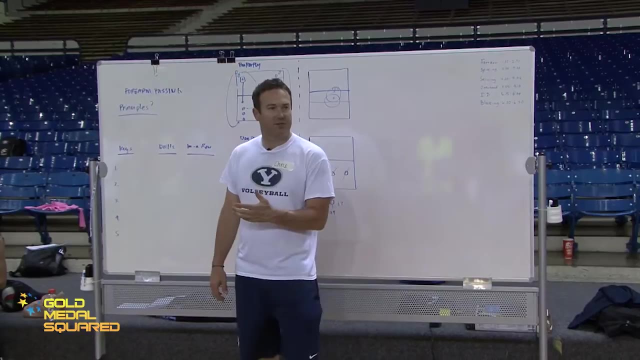 What else? principle wise: High ball pass. Say that again: High ball pass. Try to pass it higher. So it's interesting. one of the things that we come up against, or that you know comes up in these clinics, is coaches sometimes say we want to run a fast offense. 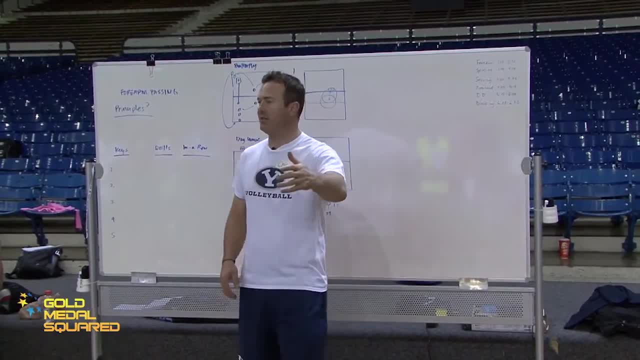 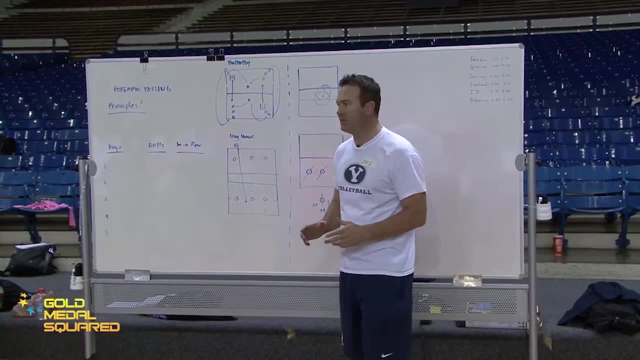 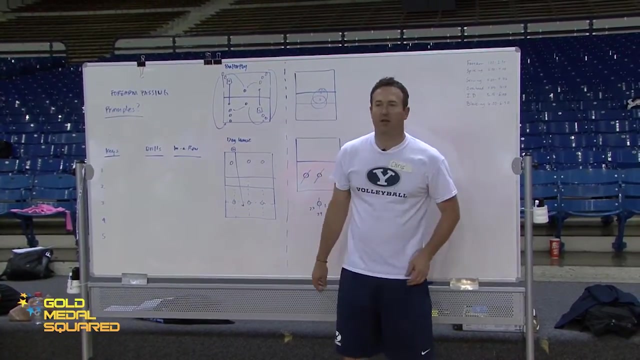 And so we want to pass fast, so we can play fast. And it turns out that we reference Brazil all the time. but they play one of the fastest offenses in the world, With their men's team just lightning fast and they don't pass fast. 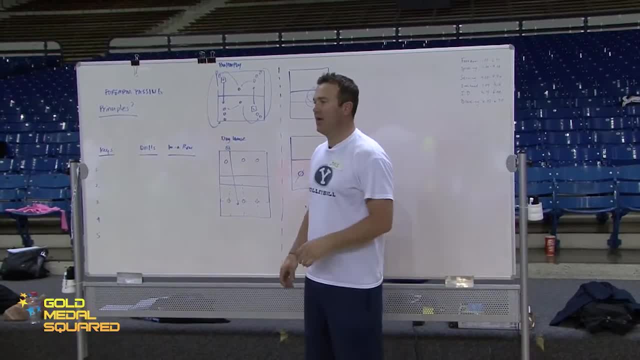 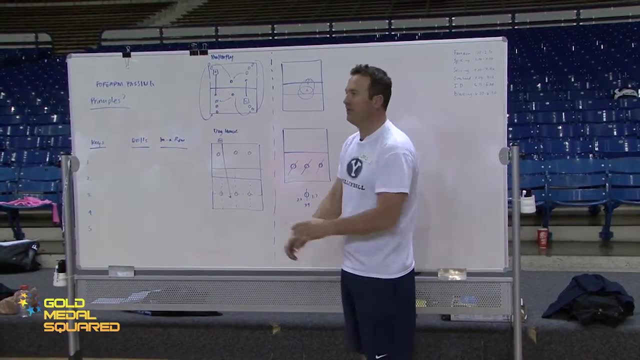 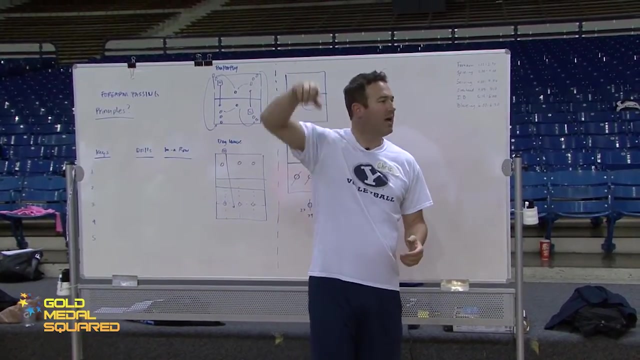 They pass as high as everybody else, And Russia, who won the gold medal in the last Olympics for the men. you'll watch them and if any time they get out of system where it isn't exactly perfect what they want, the ball ends up just going way up in the air. and you wonder, boy, I thought these teams played fast. 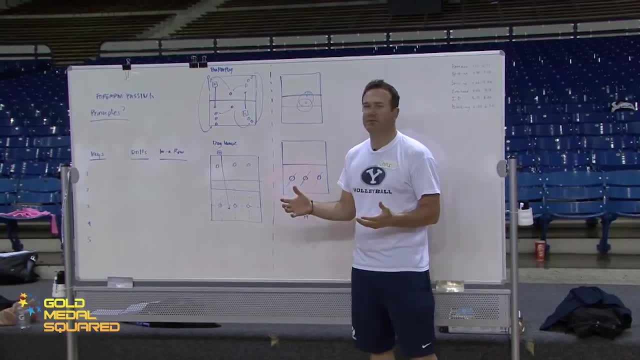 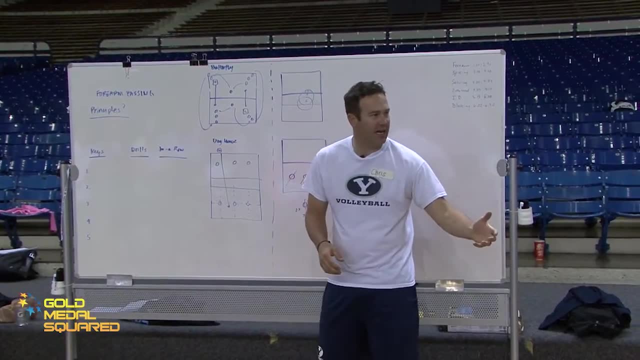 How come it's so high in the air? Well, how come it's so high in the air? Yeah, we need time to do things, and when the ball is low, it makes everybody scramble a little bit. My transition hitters are late and even in serve receive, if the ball is low, my hitters 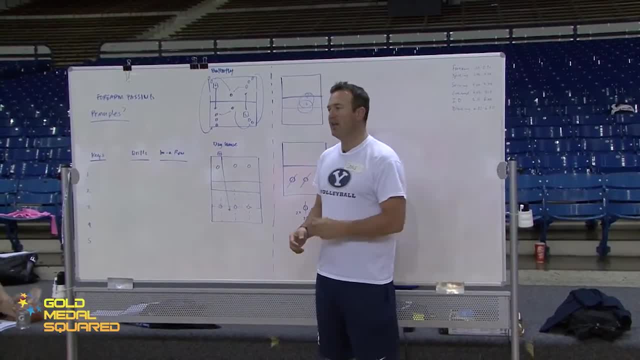 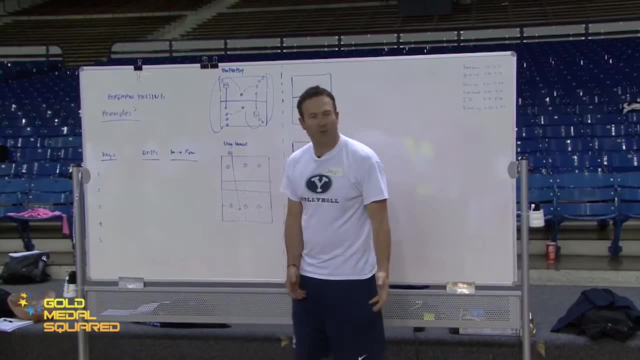 aren't in the patterns they want to be in. It's tough to control timing, And so we want passes, nice and high, so that we have time to execute everything that we want to execute. And, Brazil, you watch them, The ball goes up nice and high. 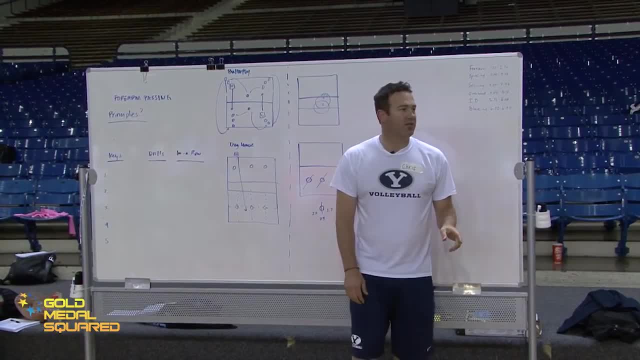 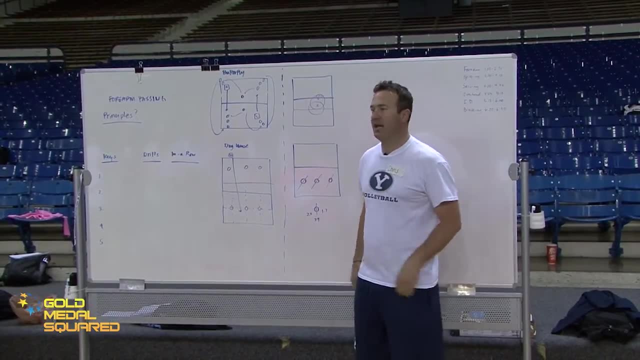 Everybody gets going and then the setter just makes it fly Once he gets the ball in his hands. that's where you go fast, Not necessarily because we pass fast. And Tom goes around and he does a lot of these camps and he was telling me: hey, one of the 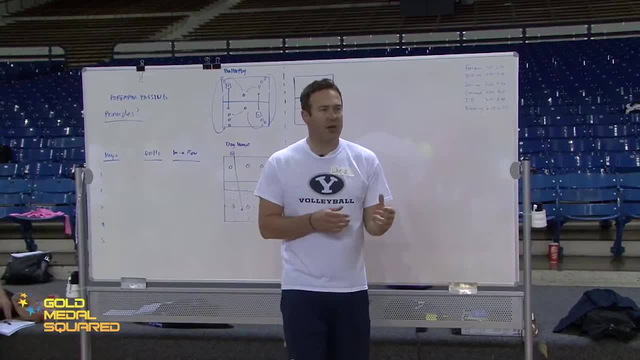 things that we do before we go to camp. quite often is we get in touch with the coach. we say: hey, what do you want to work on with your team this week? Where do you perceive their weaknesses? What can we focus on beyond what we normally do? 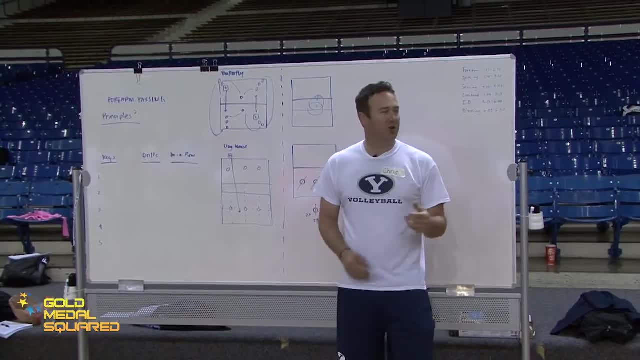 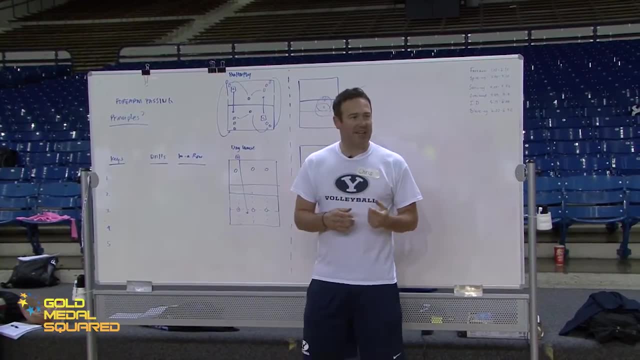 And lots of coaches will say, hey, we'd like to play faster. And so Tom tells a story of going somewhere, where they went and they said, hey, what do you want to do? And they got there and Tom was there and he said: what you really want to do is you want? 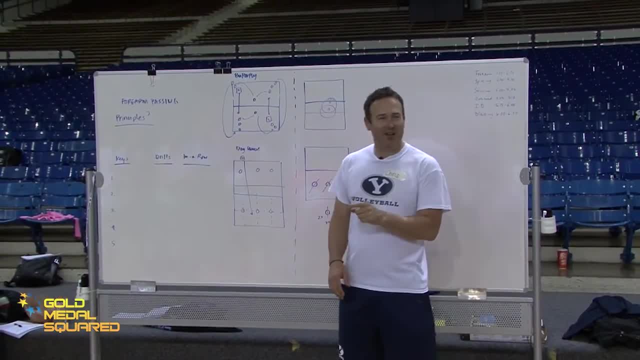 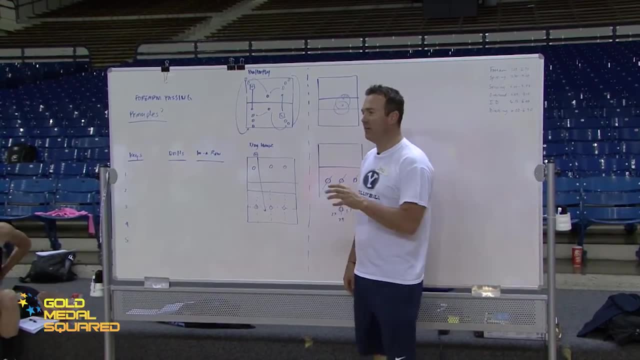 to play slower. actually, You're not good enough with your hitters and you're not good enough with your setters and you're not good enough with your passers to play as fast as you're currently trying to play, And so they were trying to get them to go slower always, so not necessarily faster is.